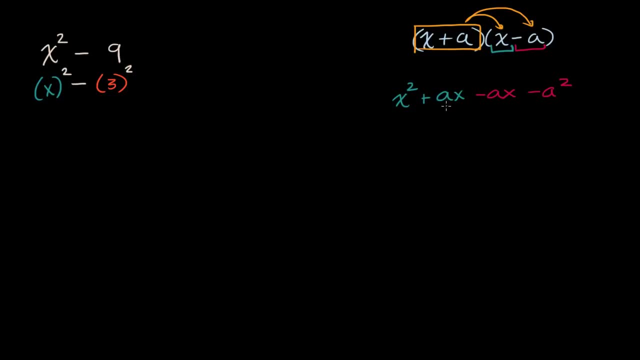 So these middle two terms cancel out And you are left with x squared minus a squared. You're left with a difference of squares: X squared minus a squared. So we have an interesting result right over here: That x squared minus a squared is equal to: 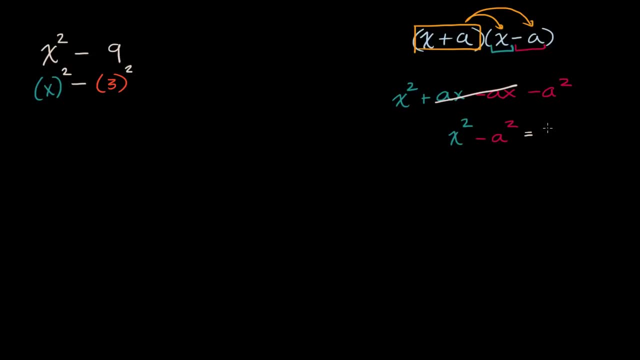 is equal to x plus a, x plus a times x minus a, And so we can use- and this is for any a, So we could use this pattern now to factor this Here: what is our a? Our a is three. 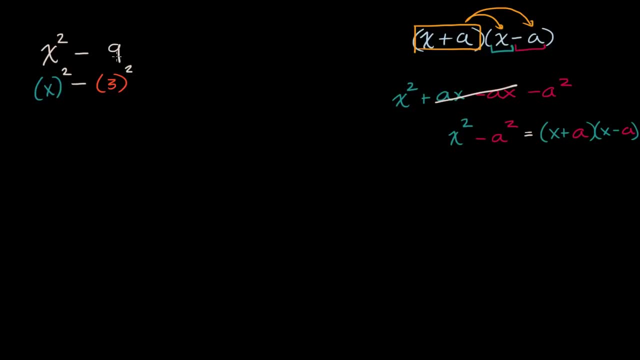 This is x squared minus three squared, Or we could say minus our a squared. if we say three is a, And so to factor it, this is just going to be equal to x plus our a, which is three times x minus our a, which is three. 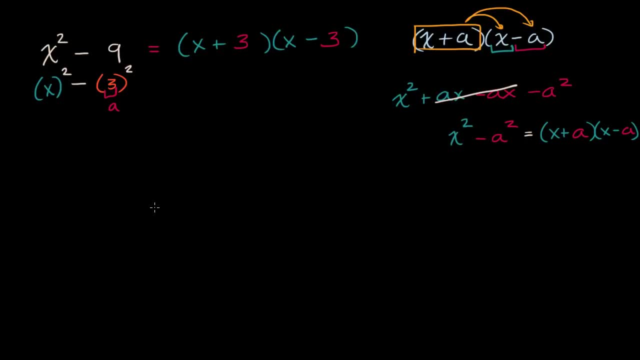 So x plus three times x minus three. Now let's do some examples to really reinforce this idea of factoring differences of squares. So let's say we want to factor, let me say, y squared minus 25.. It has to be a difference of squares. 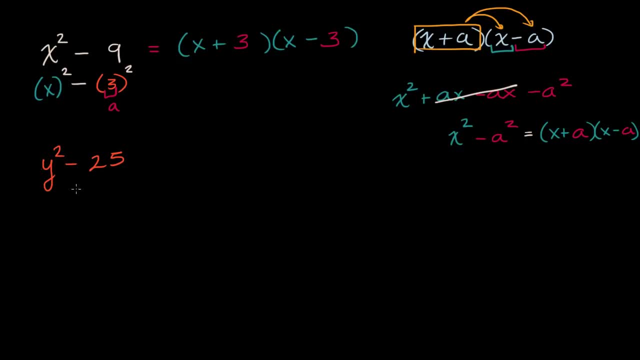 It doesn't work with a sum of squares. Well, in this case, this is going to be y and you have to confirm: okay, yeah, 25 is five squared and y squared is well, y squared. So this is going to be y, plus something. 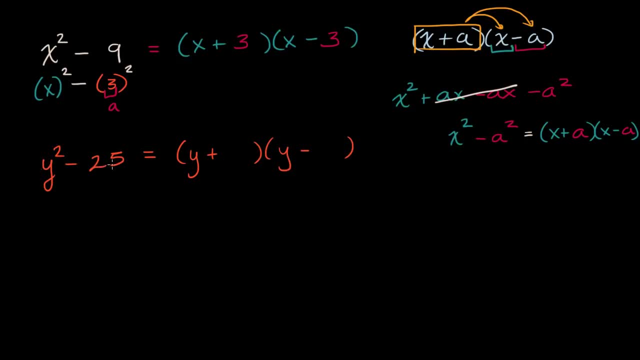 times y minus something. and what is that something? Well, this right here is five squared, so it's y plus five times y minus five, And the variable doesn't have to come first. We could write 121 minus. I'll introduce a new variable: minus b squared. 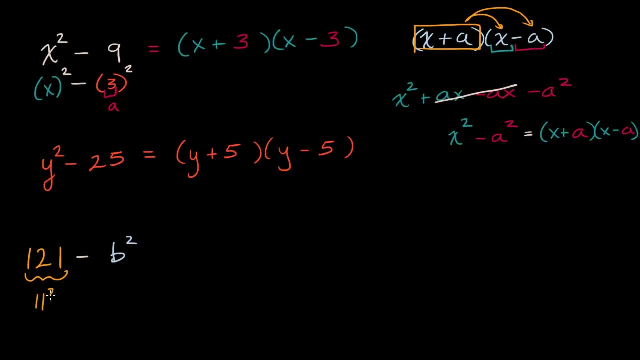 Well, this is a difference of squares, because 121 is 11 squared, So this is going to be 11 plus something times 11 minus something, and in this case, that something is going to be the thing that was squared. So 11 plus b times 11 minus b. 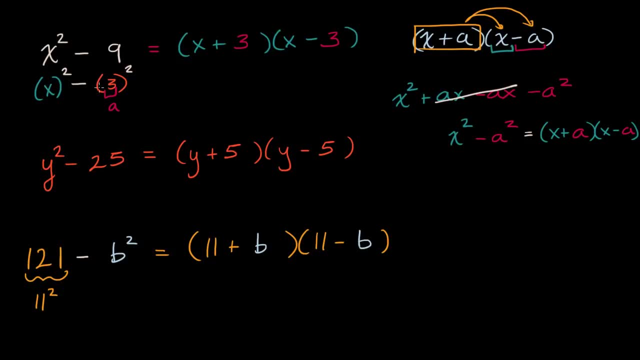 So, in general, if you see a difference of squares, one square being subtracted from another square, and it could be a numeric perfect square or it could be a variable that has been squared that you could take the square root of, well then you could say, all right,